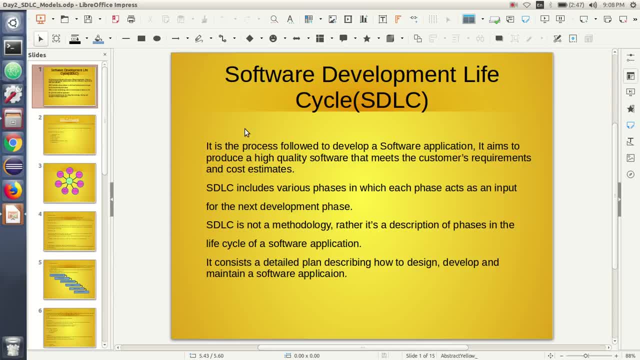 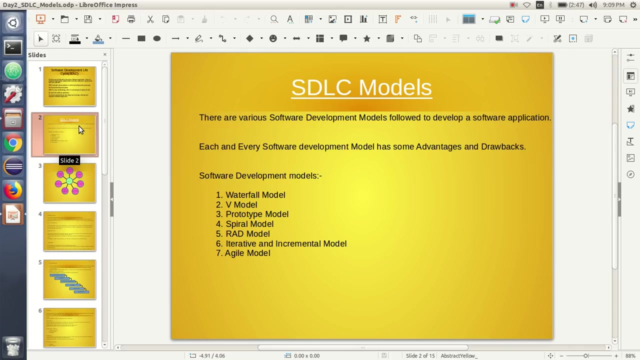 application. It consists a detailed plan describing how to design, develop and maintain a software application. So let's move to the various development models. So we have the following different software development models like Waterfall model, V model, Prototype model, Spiral. 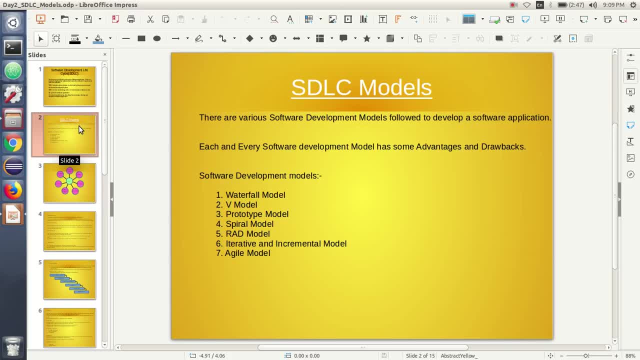 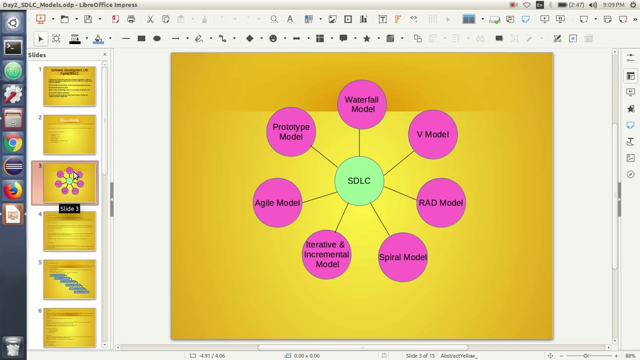 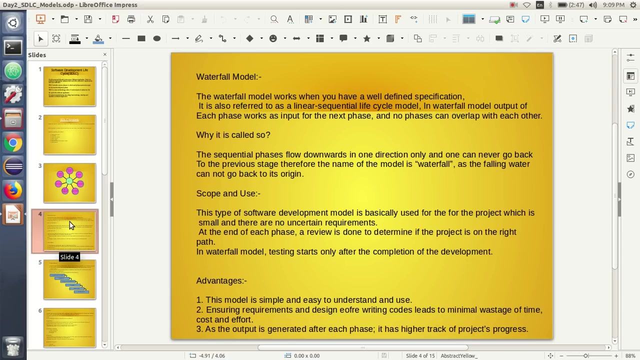 model, RAD model, that is, RAD, application development model, Iterative and incremental model, and the Agile model. So, guys, these are the most important software development models that are used in the industries nowadays. Let's start with Waterfall model. Waterfall model is the oldest model of software development. 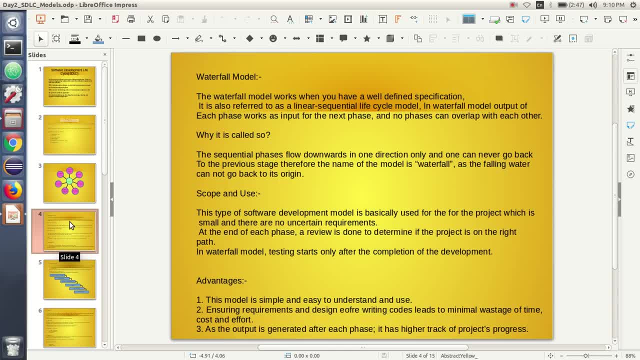 The Waterfall model works when you have a well-defined specification, and it is also known as a linear sequential life cycle model, In which, in output of a particular application, you have to have a specific specification. So you have to have a specific specification. 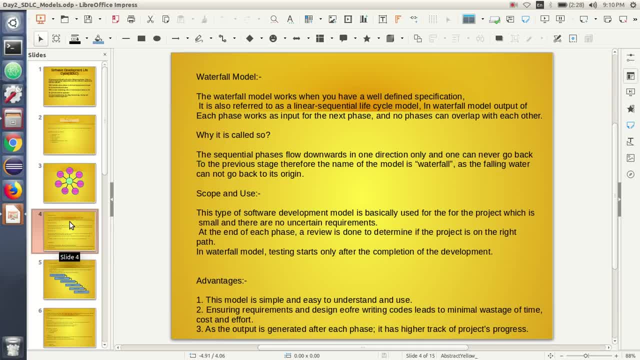 When you complete a particular phase, you have to have a specific specification or a inicetive. In that case, at any stage, you will need to complete a particular phase. So you will need to have a particular stage. So let's consider the second stage. 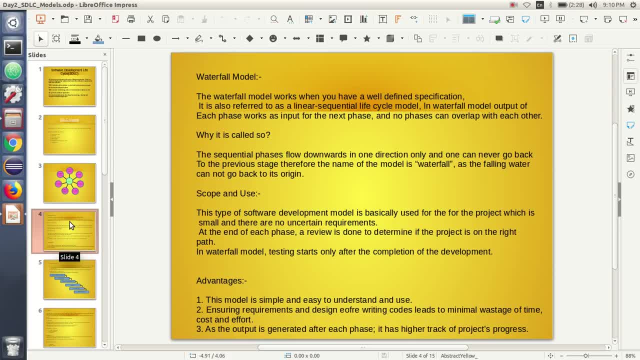 The second stage is a sequential phases. We can say that without completing a particular phase, we cannot move on to the next phase of the development model. Why it is called so? It is a sequential phases flow process, Because the sequential phases flow downwards in one direction only and one can never go back to the previous stage. Therefore, 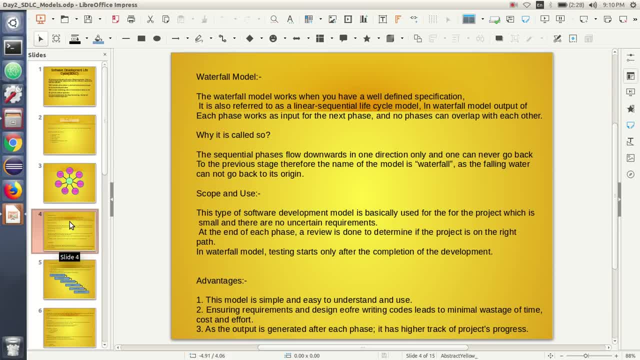 name of the model is waterfall, as the falling water cannot go back to its origin again. let's understand what are the scope and uses of using soft water waterfall model. this type of software development model is basically used for the project, which is small and there are no uncertain requirements. like all, the requirements should be well defined and well. 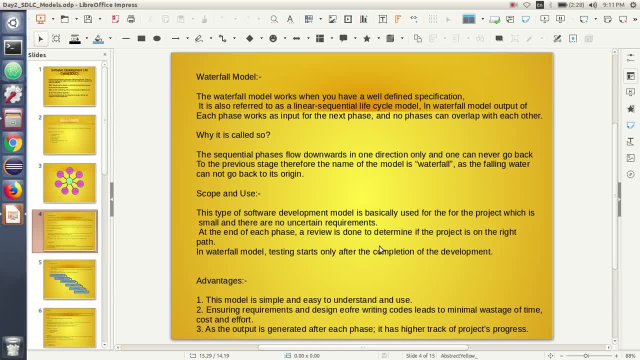 known so that that development team, development team can work on it and because it it will not allow the user or development team to make changes again in the previous phases because, as we already know that the output of a particular phase acts as an, as the input for the next phase. 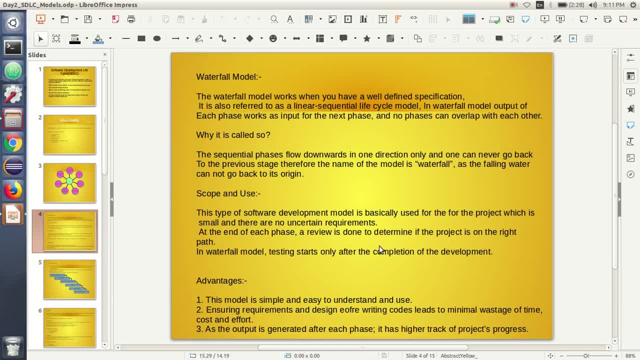 okay. so in waterfall model, testing starts only after the completion of the entire development, and at the end of each phase a review is done to determine if the project is on the right path or not. let's understand the advantages of using waterfall model. so, guys, this is this. 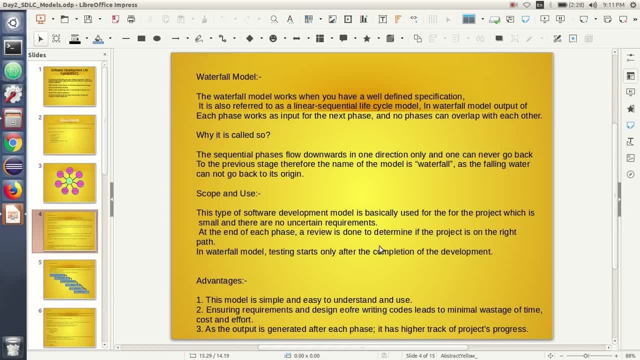 model is simple and easy to understand and easy to use and it ensures the requirements and design before writing codes, leads to minimal wastage of time and cost efforts. so as the output is generated after each phase, it has higher track of projects progress so we can easily track the track that, whether we are our, we are accomplishing the project phases on right time. 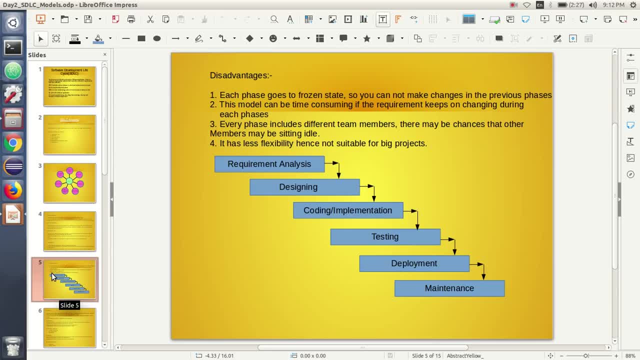 or not, or, like the time estimates are meeting its deadline or crossing its deadline, so we can easily track all these these things in the waterfall model. so, guys, let's discuss the disadvantages of waterfall model. the disadvantage of waterfall model is like: each phase goes to the frozen state, so you cannot change. 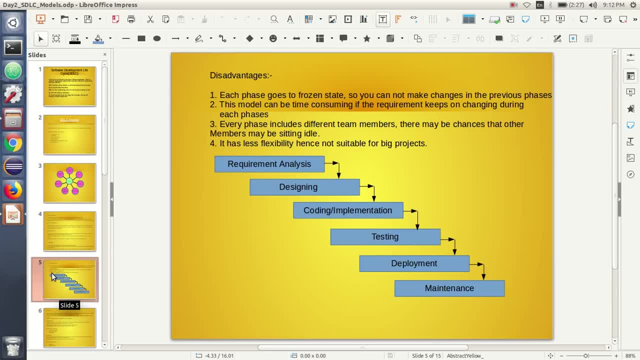 you cannot make changes in the previous phases, like you have the designing phase. if you have designed the application, then you can after the, during the implementation phase. if you come to know that you have to make some changes in the previous stage, like in designing stage, then you 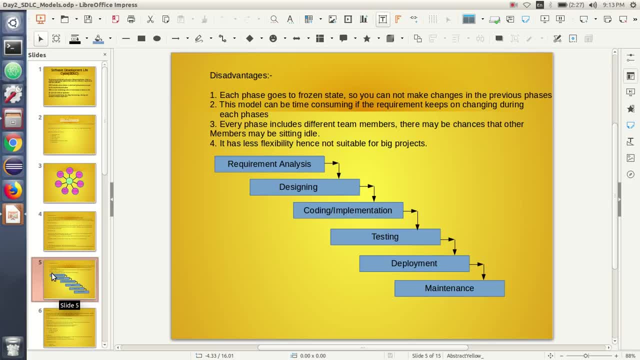 cannot go back to the designing phase to make changes. so this is the most important thing to. so this is the most uh, we can say that this is the biggest drawback of using waterfall model: that it is not adaptable and it is not flexible, that user cannot make changes in the previous. 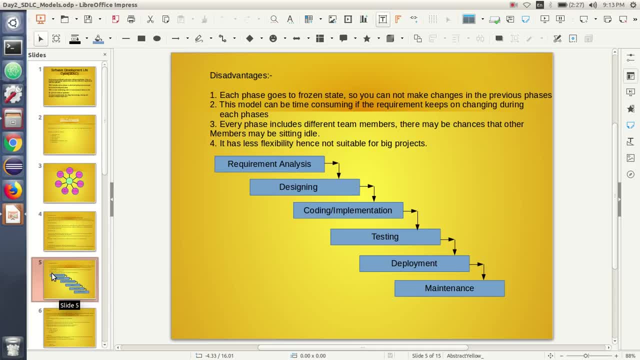 stage of the development life cycle. okay, this model can be time consuming if the requirement keeps on changing during each phase. like suppose we are in the designing phase and the user want to want to add or remove some of the features, or that may affect the designing also. like suppose we have a website. 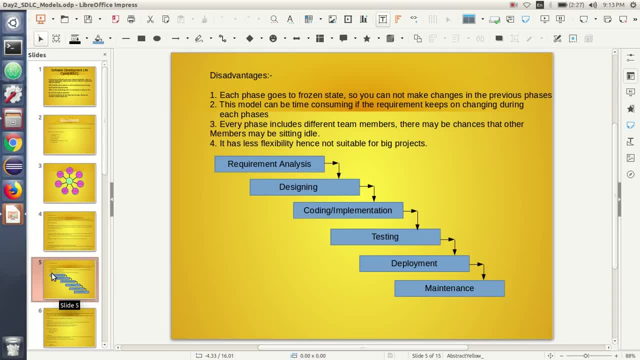 and we have a web page and that contains, uh, 10 or 12 fields and while designing the web page, we came to know that the customer wants something else. in the designing process, designing feels like we want to add more fields in the webpage, so it will take some time and, uh, it is like a 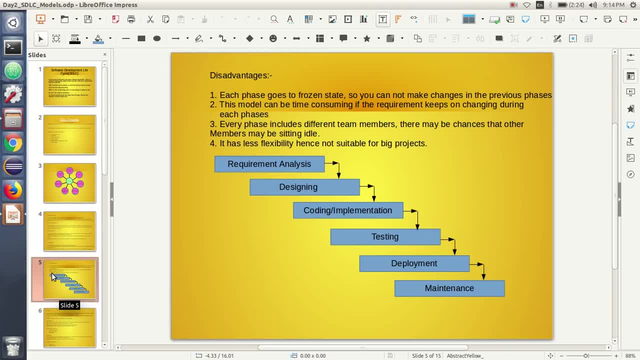 very time consuming process because without making changes in the designing phases we cannot move on to the coding phase of the development. so it is time consuming as well. so every phase includes different team members. there may be chances that members may be sitting idle, like as we know that. 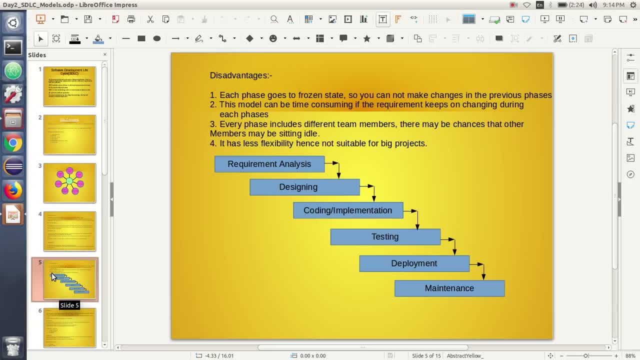 each, each phase or each process have some other team, like designing. designing team is different from coding team or the development team, like we all have ui or ux team or designing team and coding team and testing team. so so it may be, there may be possibility that if you have only one, 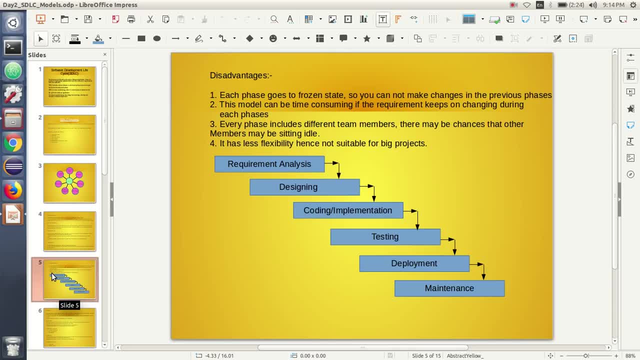 project at that time, then the if the development team is working on designing, then it may be possible that the coding team is sitting idle, so you cannot utilize all the resources simultaneously. so this is also the biggest drawback of waterfall model, and it has very less flexibility, hence not suitable for big projects. 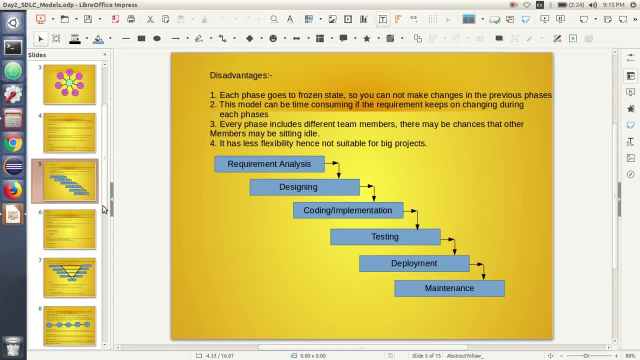 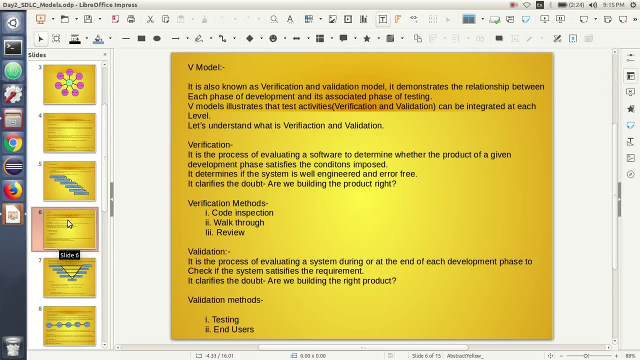 okay, so let's move on to the next, next development model. okay, so next model is v model. it is also known as verification and validation model. it demonstrates the relationship between each phase of development and its associated phase of testing. v model illustrates that test activities like verification and validation can be integrated at each level. 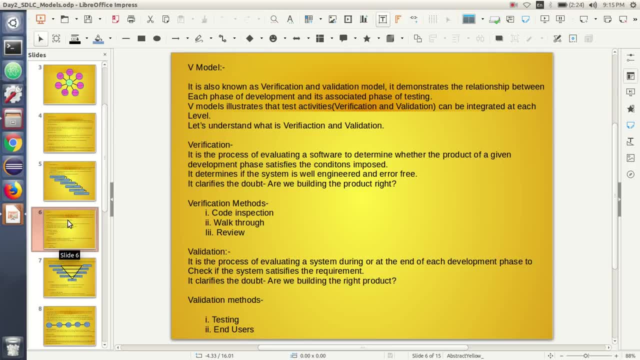 okay, before moving further and understanding what is v model, let's understand the concept of verification and validation, indeed, so that it will be easy for us to understand the whole process on the whole model easily. so, guys, verification is the process of evaluating a software to determine whether the product of a given development phase satisfies the conditions imposed. 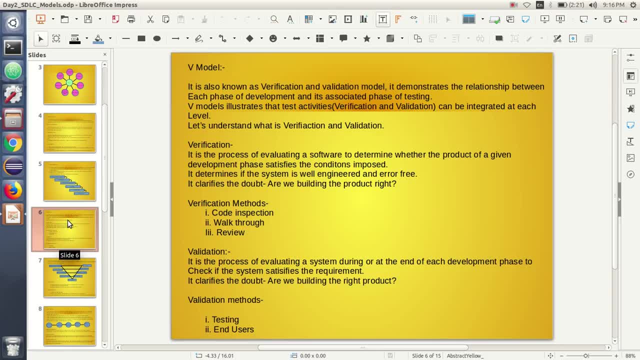 or not. it determines if the system is well engineered and error-free. it clarifies the doubt that: are we building the product right? like verification is a process that is done in each phase, and there are various methods of verification as well, like code inspection and walkthrough, and 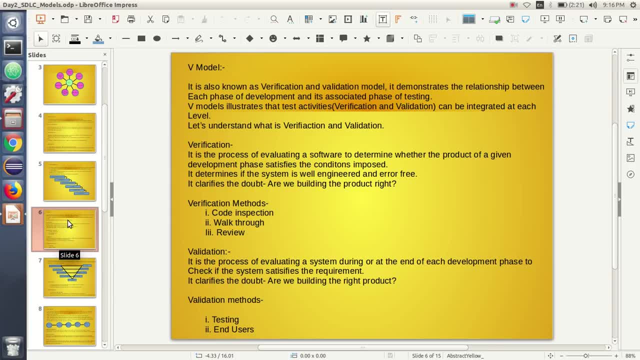 review. all this comes under verification process. what is validation? it is the process of evaluating a system during or at the end of each development phase to check if the system satisfies the requirement or not. it clarifies the doubt: are we building the right product? so, guys, you have to understand. 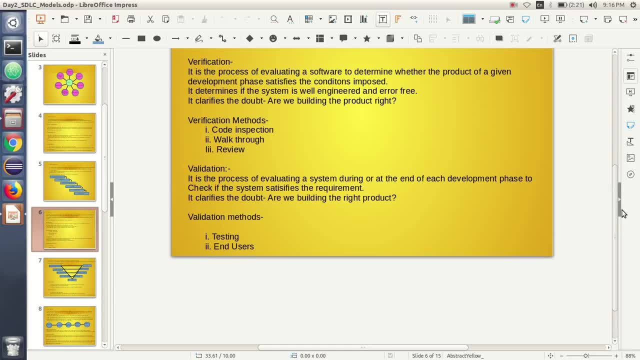 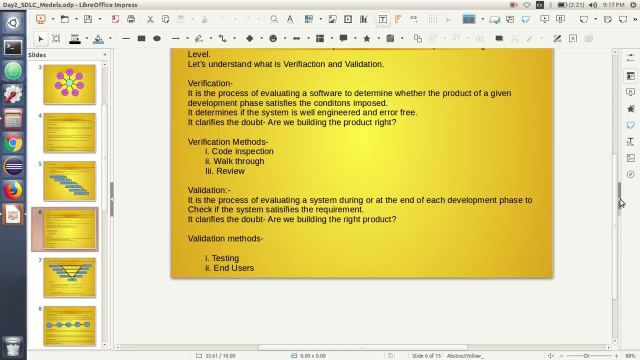 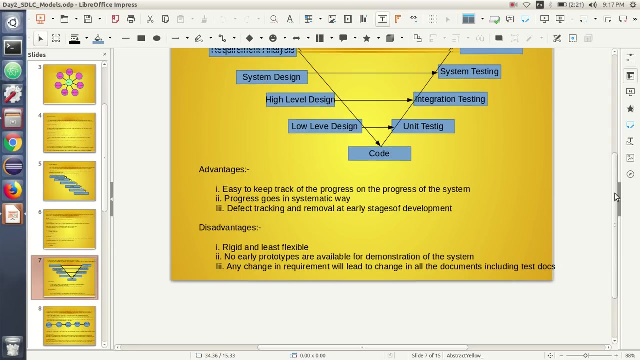 the concept of verification, validation. so we can say that validation is the process that that is carried out after the completion of a particular phase and verification is the process that is carried out during a particular phase. so where the validation methods includes testing and end users, like you can say that uh u8 of an application also comes under validation process. 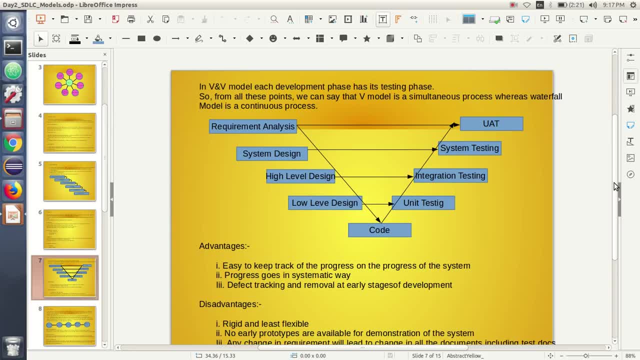 in vnv model, each development phase has its testing phase. so from all these points, we can say that the testing is carried out in vnv model is a simultaneous process, whereas waterfall model is a continuous process. like in waterfall model, testing is carried out after the completion of 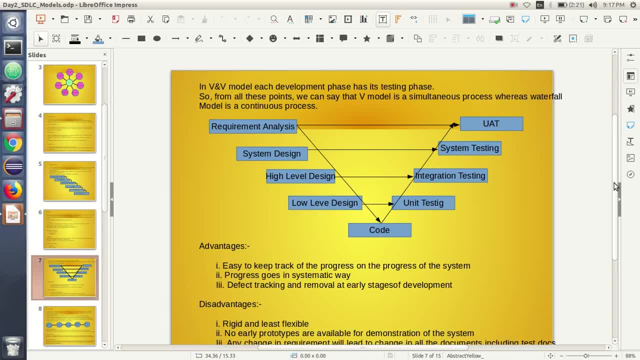 all the phases, but in v model we can simultaneously do the testing of the application as well, like for low level design. for high level design, for system design, we have the simultaneous testing process. also like for low level design we have, and for high level design we have integration testing. and for system level design. 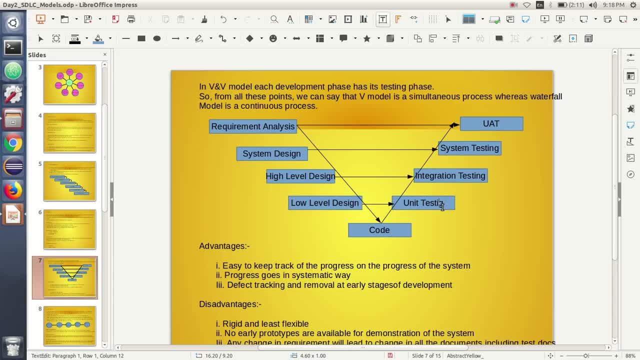 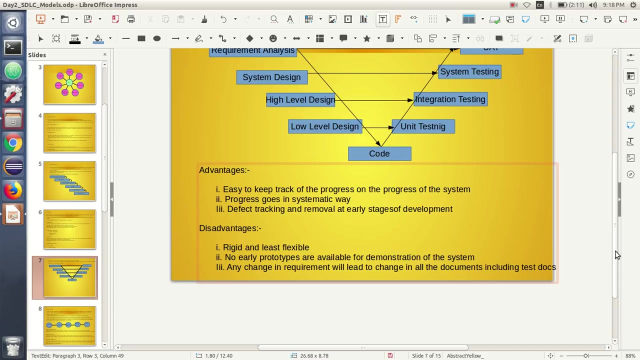 we have system testing. so, and for the evaluation or of requirements, we have u8, like user acceptance testing. okay, so let's understand the. what are the advantages and disadvantages of vnv model? so, guys, the advantages of v model includes that it is easy to keep track of the progress on the. 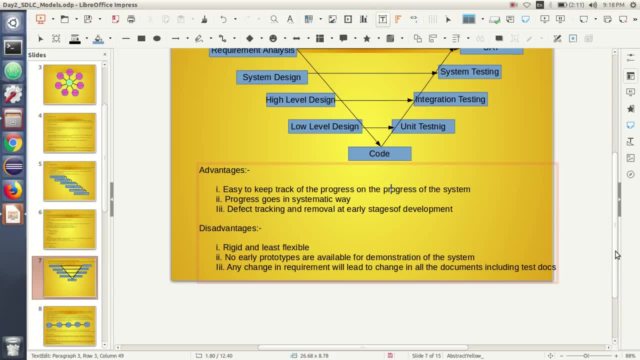 progress of the system. like uh: how much the task is completed, how much of the requirement is fulfilled. in vnv model the process goes in a systematic way, like uh: after the low level design, we go for the unit testing, high level design, we go for the integration testing. so it's 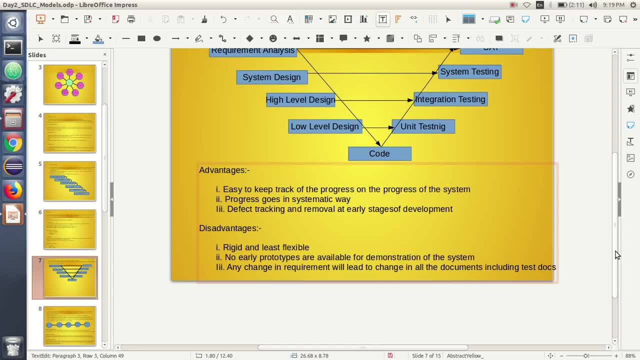 a very systematic way of application testing and after the low level level testing we go for the application development and in remodel, defect tracking and removal at early stage of development is possible. so it is very uh, we can say that the application which we are developing right now, 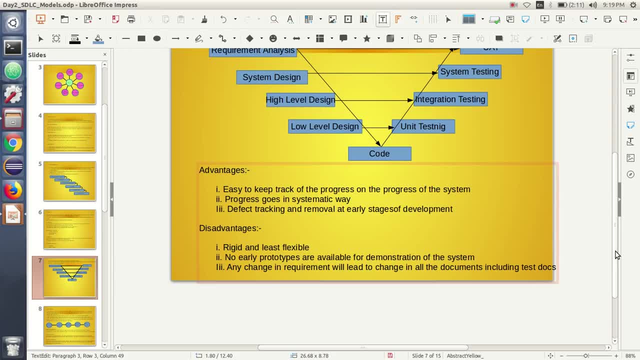 is going to be bug free at a particular extent, like because we are following the testing as well. for each and every uh, each and every stage of development, like for all the, all the development steps, like low level design and high level design, we have the test corresponding testing method. 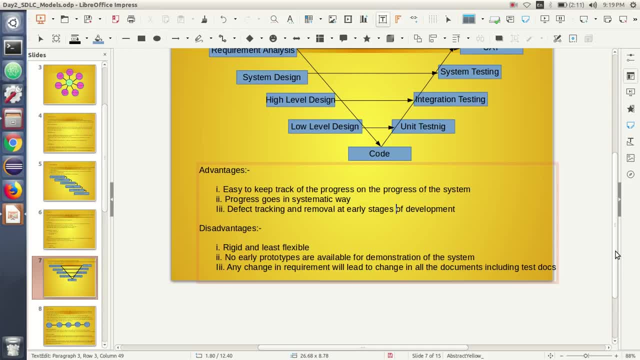 also and the disadvantages of vng model inputs: like it is rigid and least flexible. like it is not up to that flexible. like changes cannot be implemented again and again. and no, uh, no early prototypes are available for that demonstration of the system. like prototypes are not available for showing the demo to the client because we have all the 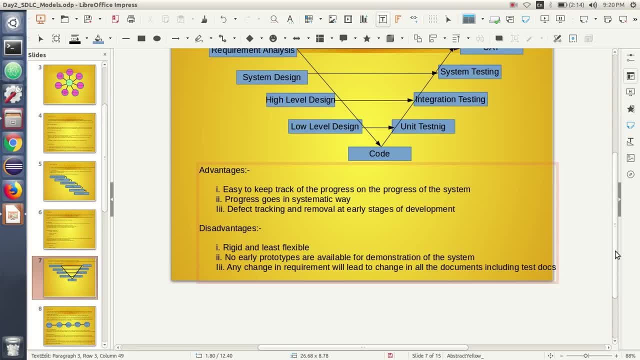 process of development in like. it follows a systematic way of development like low level design and high level design and system design. any changes in the requirement will lead to change in all the documents, including testing documents also. so it's the. you can say that it is the. 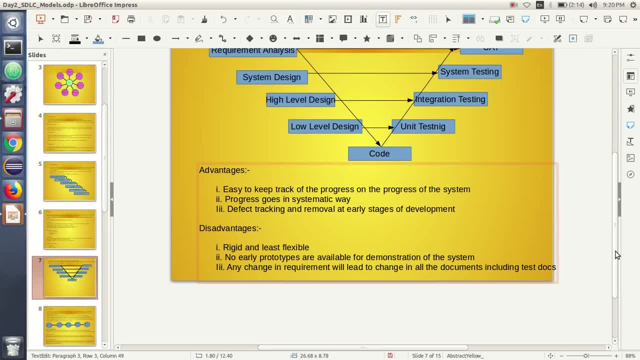 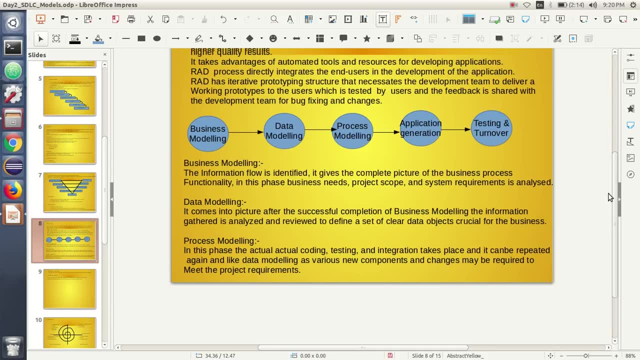 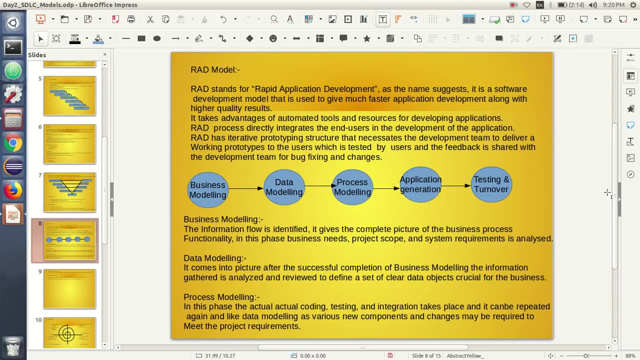 biggest disadvantage of of vnbd model, you guys. let's move on to the next model, which is red model. that is, rapid application development. as the name suggests, it is a development model that is used to give much faster application development, along with higher quality results. it takes advantages of automated tools and resources for developing application. 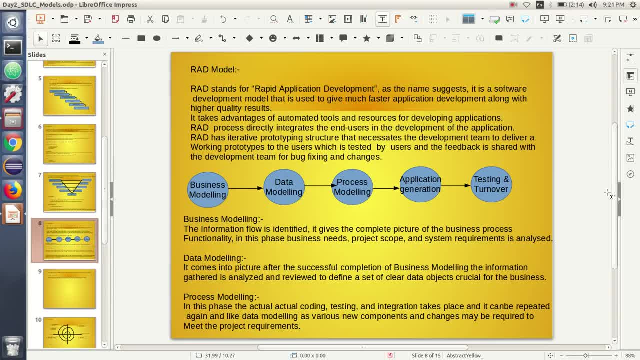 and red process directly integrates the end users in the development of the application, and rad has iterative prototyping structure that necessitates the development team to deliver a working prototype of prototype to the user, which is tested by users and the feedback is shared with the development team as well for the fixing of bugs and all the changes that are proposed in the 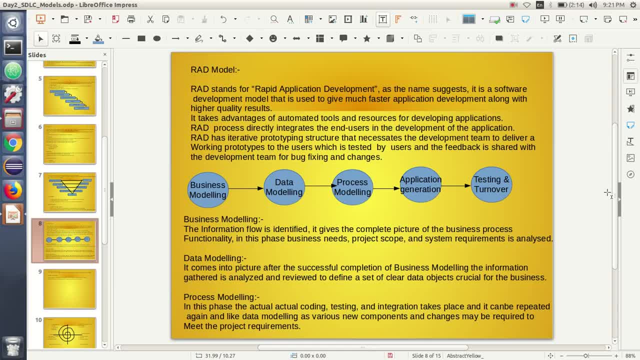 on that particular prototype. uh ran model follows a process of business modeling and data modeling, followed by process modeling, application generation and testing and turnover. so let's understand what is business modeling, business modeling, uh, in this uh we, the information flow is identified. it gives the complete picture of the business process. functionality in the functionality in this phase. 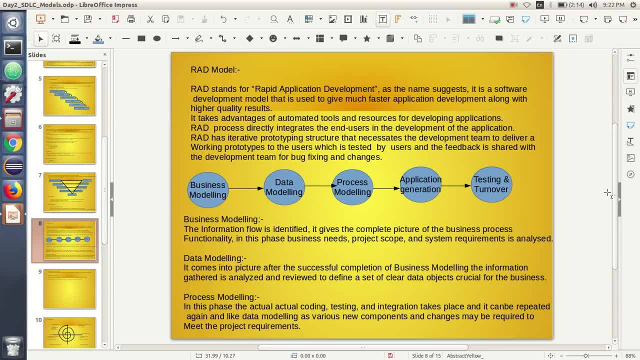 business needs, projects, scope and system requirements is analyzed, we can simply say that in business modeling we can. we can prepare the brs of that application like business requirement specification that that will define the scope and objective of that application in the data modeling process. it comes into picture after the successful completion of business modeling where the 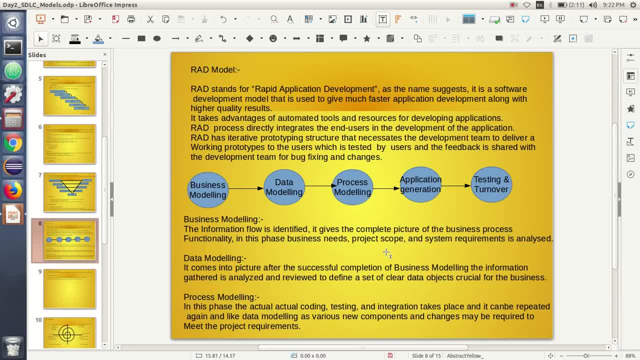 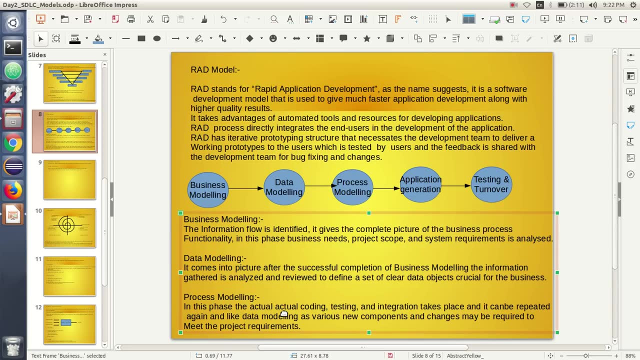 information is gathered and is analyzed and reviewed to define a set of clear data objects crucial for the business, and in the process modeling phase, the actual coding, testing and integration takes place, and it can be repeated again and again, like data modeling, as very variously components and changes may be required to meet the project. 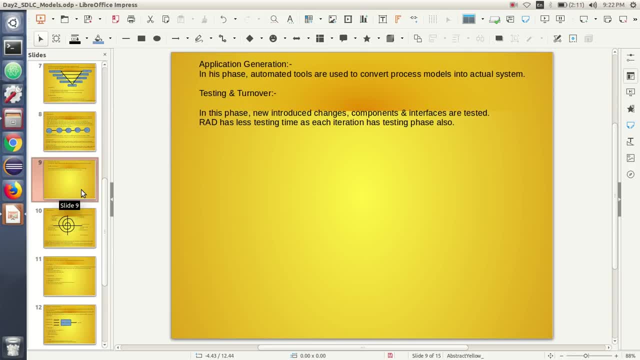 requirements. in the application generation phase, the automated tools are used to convert process models into actual systems, and in the testing and turnover phase, new introduced changes, components and interfaces are tested. so red has less testing time, as each iteration has testing phase also. so that is why it is it is called rapid application development, like 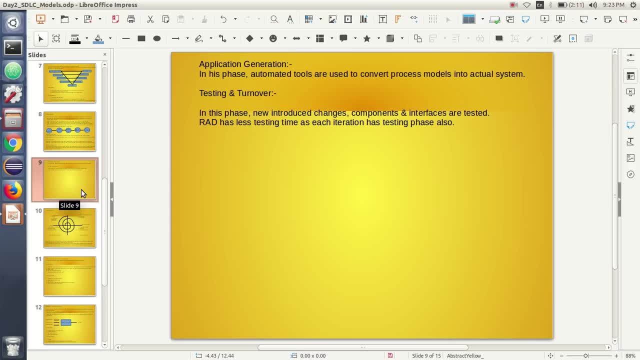 all, there are set of automated tools that are that are used for the application development, and each has its own testing time. so it has a collectively we can say that it has a less testing time because for each iteration, because each phase has its own testing time. so that is why it is also 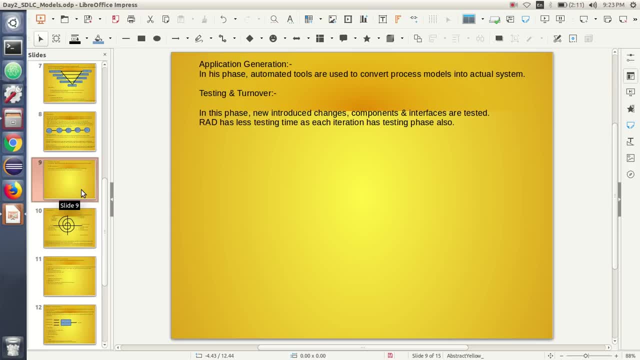 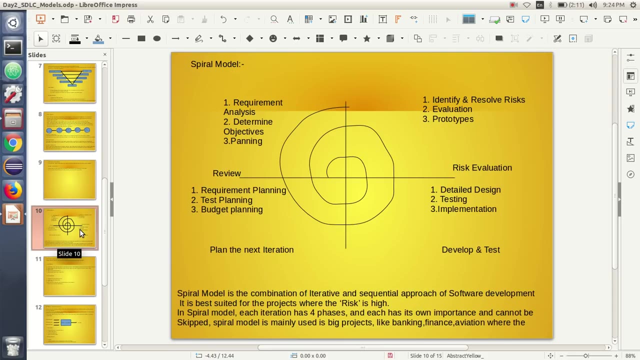 called rapid application development because, as we know, that most of the time of the application development is consumed in the testing process. so that's why it is called rapid application development. friends, we have next model, which is a spiral model. it is in the form of, like, it has a various continuous circular process and it has 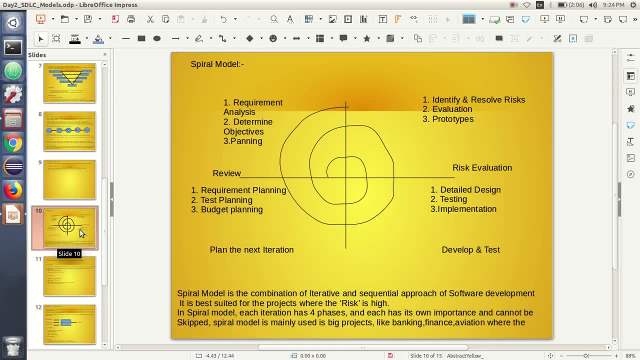 it is the combination of iterative and sequential approach of software development. it is it is best suited for the projects where the risk is very high. like each iteration has four phases and each has its own importance and cannot be skipped, it is used for big projects where the risk is very high and like banking projects, finance projects, aviation projects. 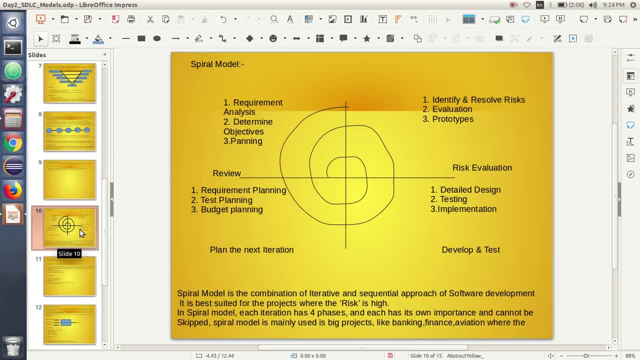 where the success depends on the risk analysis of the application. so, guys, if we talk about risk, then we can analyze the risk only if we have the expertise of that person. so that is our next step of that particular domain. like, if we we don't have sufficient knowledge of a 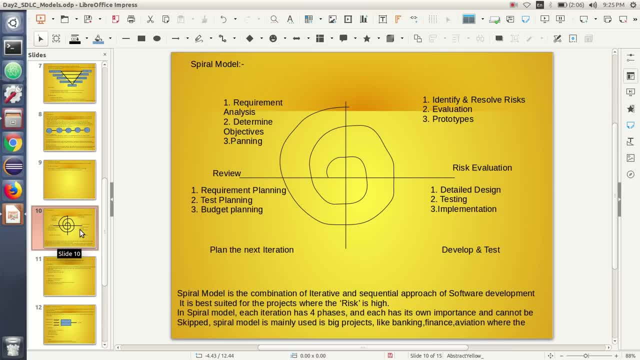 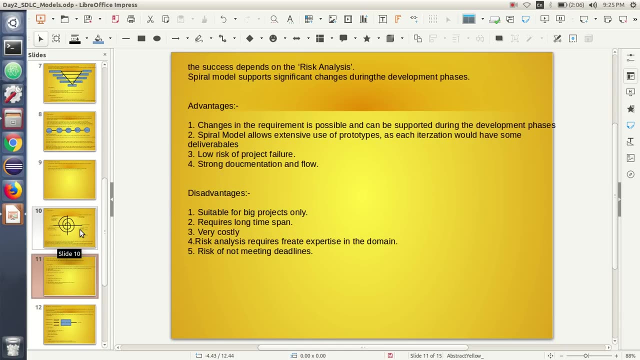 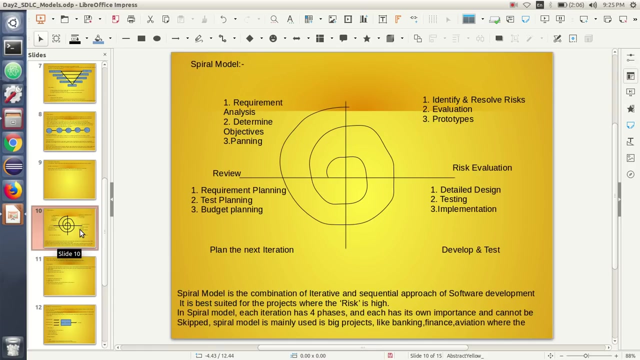 particular domain, then we cannot identify the risk, of the risk that can occur or that can occur in near future. so it requires a lot of expertise of that particular domain in which we are going to build. that application spiral model supports significant changes during the development phases, so as we 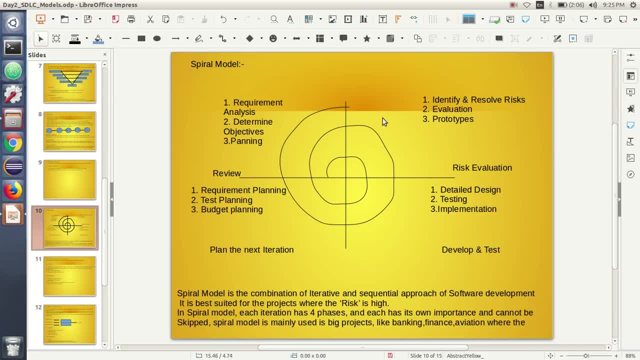 can see that it is a circular model where that is, starts with the requirement, analysis and determining objectives and planning and followed by the identification and resolution of risk, evaluation and preparing prototypes and after that detailed design and testing of the prototype is implemented and then again we plan the next iteration and budget planning for the next iteration and next. 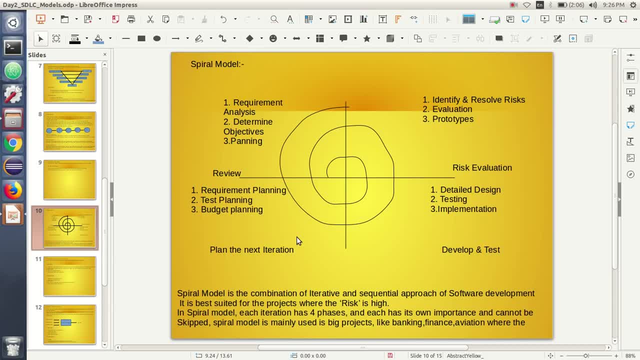 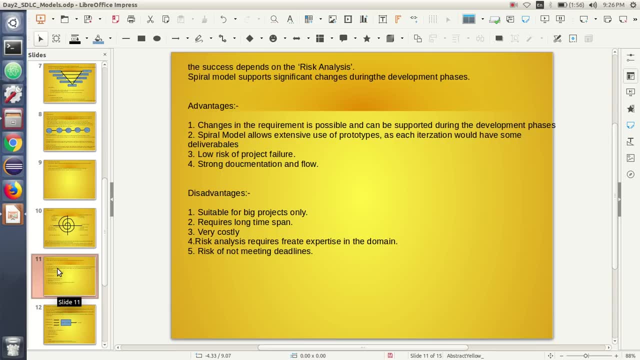 deliverable that that will include some changes or some bug fixes. okay, so let's understand what are the advantages and disadvantages of using spiral model. so the changes in the requirement is possible and can be supported during the development phases. spiral model allows extensive use of prototypes, as each iteration would have some deliverable. the risk of project failure is. 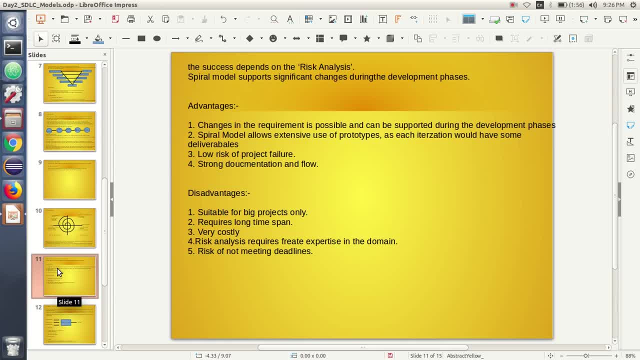 very low because, as i just talked about this earlier, like the, you must have that level of expertise in that domain so that you can analyze the risk of that project. so it's obvious that someone who is going to analyze the risk of that application must have that expertise. 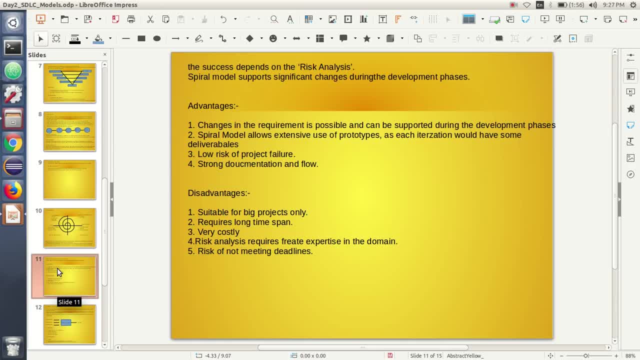 that's why the risk of project failure is very low here and it requires a strong documentation process and flow of the application. what are the disadvantages? so it is suitable for big projects only and requires a long time span. like, as i told you, that it is a continuous process and sequential. 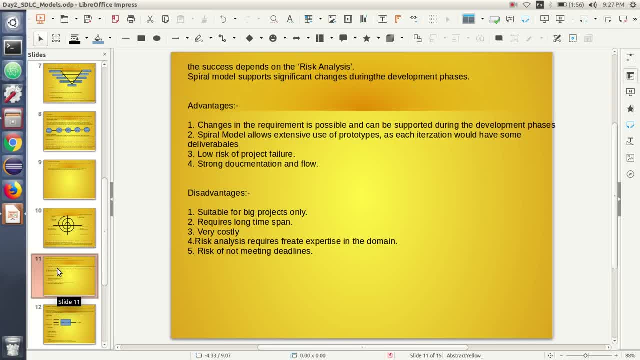 so it needs a very long time span where user needs to wait for the iterations and the deliverables that are going to be deployed after a particular iteration, and it is very costly and, as i told you, that it requires a very great expertise in that particular domain. so 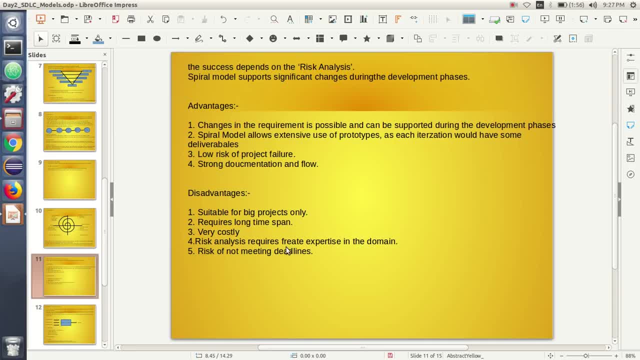 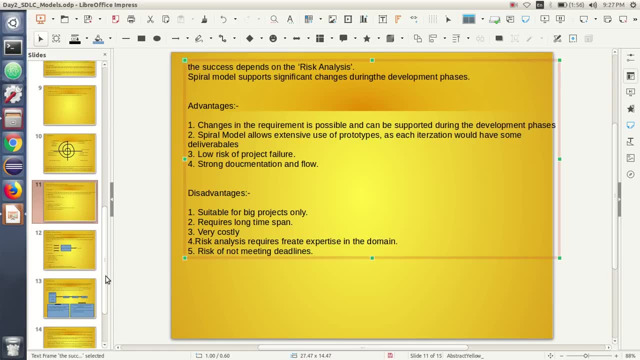 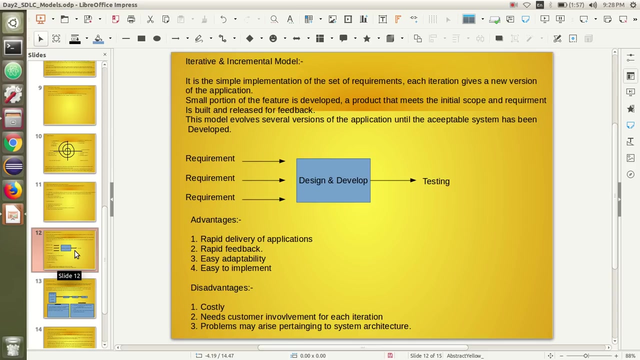 and there may be chances of like not meeting deadlines, like maybe sometimes the deadlines will be crossed and the deliverables are not available for deploying to the clients. so these are the disadvantages of spiral model. let's discuss the iterative and incremental model. it is a simple implementation of the set of requirements. 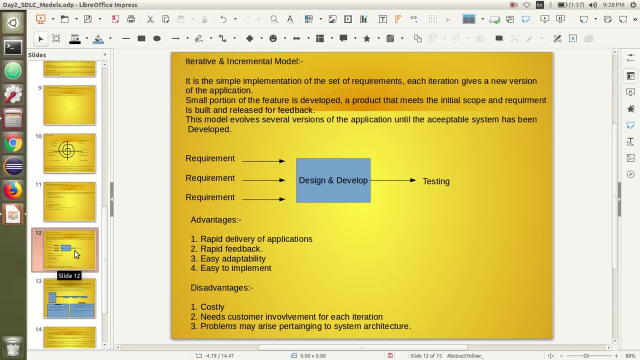 and each iteration gives a new version of the application and a small portion of the feature is developed. a particular version of the application is developed and a small portion of the feature is developed. a product that meets the initial scope and requirement is built and released for feedback. we can say that. 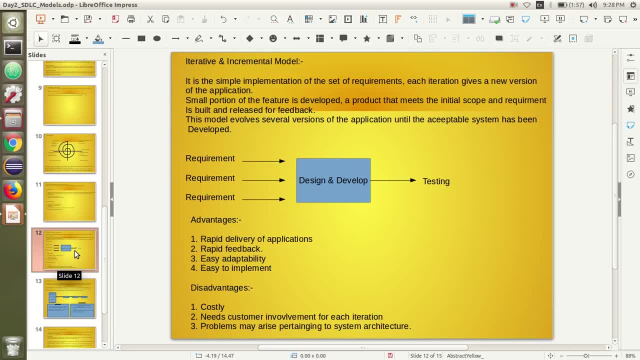 in each iteration we have a particular working application that that has all the features that were proposed in that particular iteration and is deployed to the client for for the feedback, and we can say that it is a kind of user acceptance testing where user uses his application or his prototype of that application and shares the feedback with the. 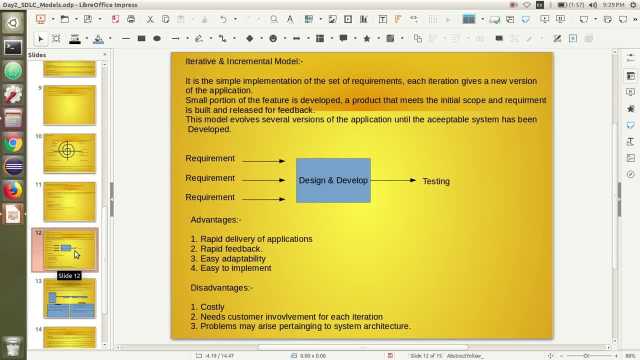 development team. so we have requirement and designing and development and then testing process. you guys, the advantages of iterative and incremental model includes rapid delivery of the application, rapid feedback, easy adaptability and easy to implement. and all these things are very important for the software development life cycle and with respect to the client as well, because 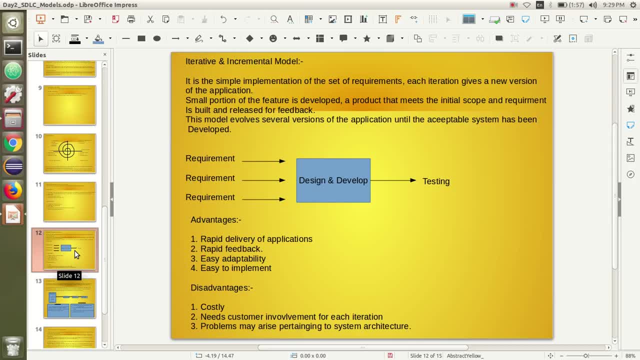 clients always want to share his feedback on the application developed. he wants that his application should be that adaptable and that flexible that it will always accept some sort of changes in the while, during the development or after the deployment of the application. and yeah, the most important thing thing is the rapid delivery of the application. 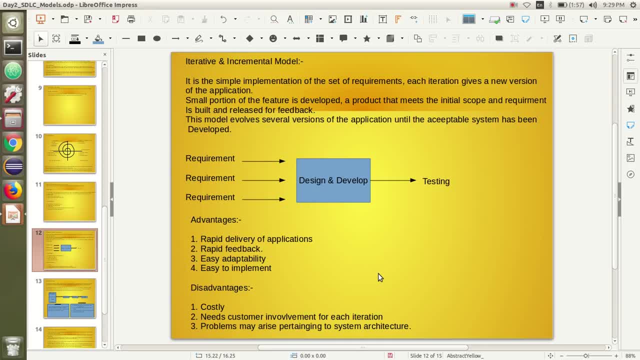 so, and the disadvantages includes: like it is very costly, so it requires customer involvement for each iteration. problems may arise pertaining to system architecture. like it may be, it may be possible that the system architecture is not up to that mark, so this may create some sort of problems. 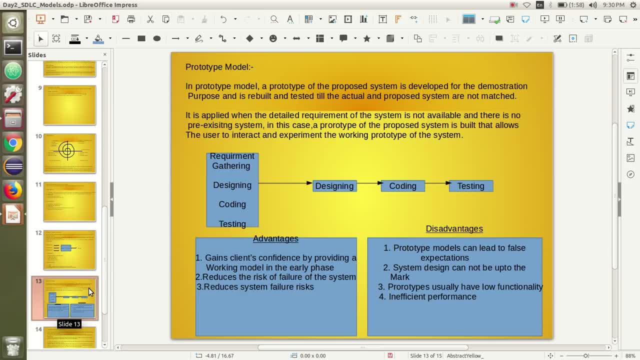 and next one is prototype module. in plot model, a prototype of the proposed system is developed for purpose and is rebuilt and tested till the actual proposed system are not matched. it is applied when the detailed requirement of the system is not available and there is no pre-existing system. 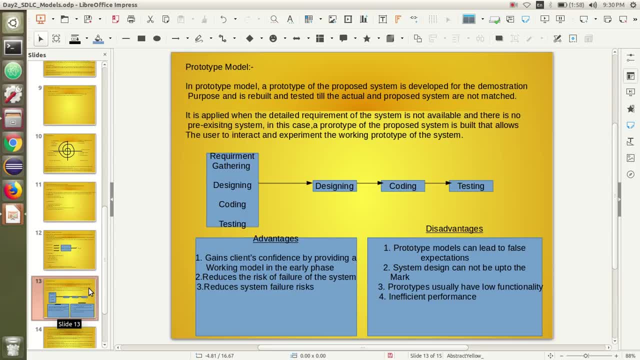 in this case, a prototype of the proposed system is built that allows the user to interact and experiment. experiment or experience the working prototype of the proposed system, as we can say that if we don't have any particular filter requirement or we don't have any fixed pre, 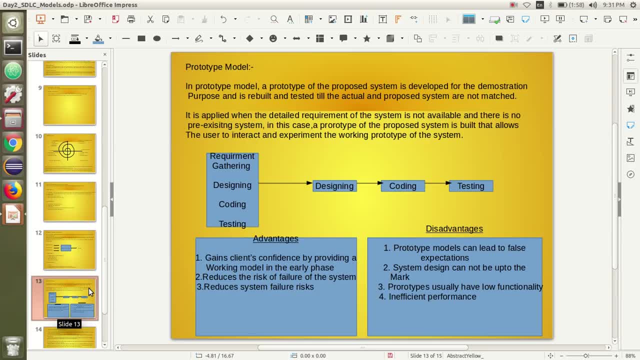 existing system, then we we built, we build a working demonst demo of that application. as for the users requirement, and we deliver it to the clients so that he can experience that how the system will work after the actual development of the proposed system. so it's a very user-friendly thing that user will. 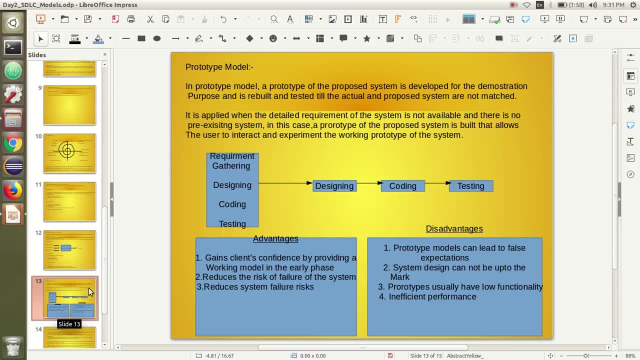 experience that how his system will work in the near future. so, guys, advantages of prototype model includes: like it gains clients the confidence by providing a working model in the early phase. like suppose a client comes to a development team and says that I have these requirements and I want this kind of application, and within the week. 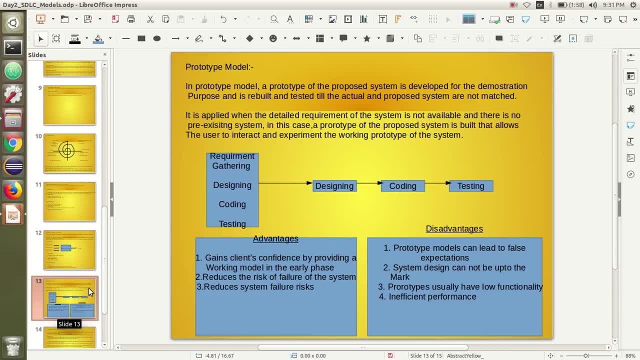 he is having a demo or he is having a prototype of the proposed system, so he will be very happy and will be, will feel like he will be very happy to use that application and will, and by this you will gain clients confidence also. Thank you, 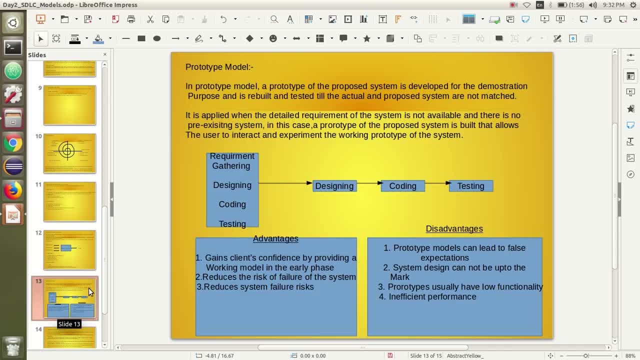 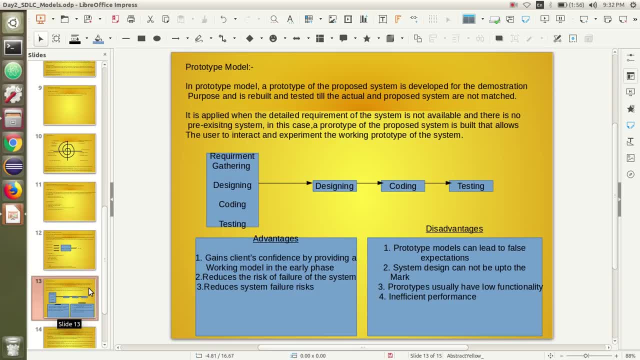 client interaction is always there and client will always have the prototype of that application So he will always share his feedback on that app: that it is up to the mark or not. it is fulfilling my, filling my requirements or not. so they are very, very small or low chances of the system failure. 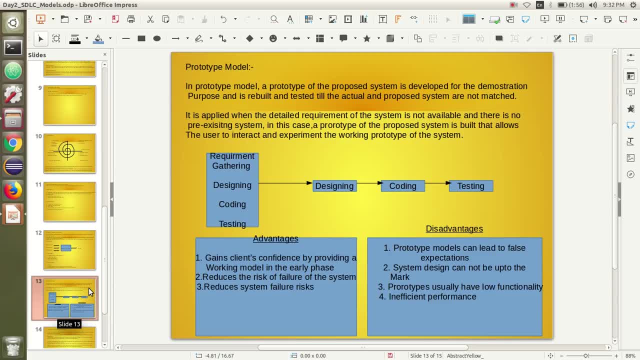 and disadvantages includes. like prototype models can lead to false expectations, system design cannot be up to the mark and prototypes usually have low functionality. like user development team can never, ever develop a prototype with all the functionalities, because it's a prototype and all the things will be implemented in each iteration and 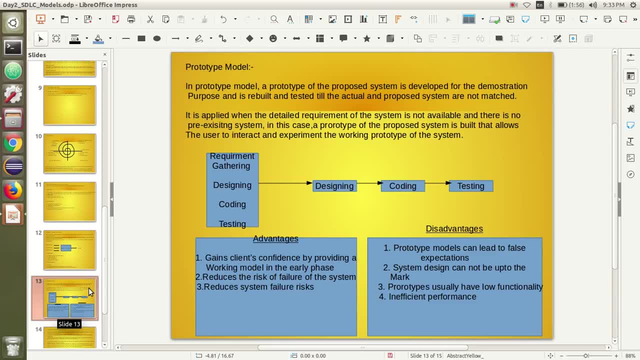 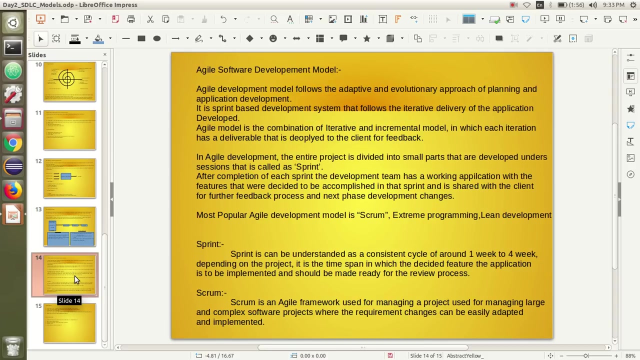 in each prototype till the actual requirements are matched. so it will have a very low functionality till the actual system is developed and maybe it is not that efficient to perform the actual operations. so these are the disadvantages. let's discuss the next software development model, that is, agile software development model. this is the. this model is in. 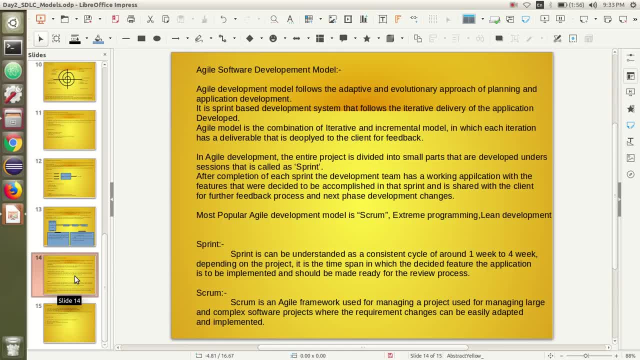 boom nowadays because it is means almost every company or every firm is using, as i, agile methodology for developing the applications because of its adaptive nature and its flexibility to accept changes. so let's discuss what is a software development model? agile development model follows the adaptive and evolutionary approach of planning and planning and. 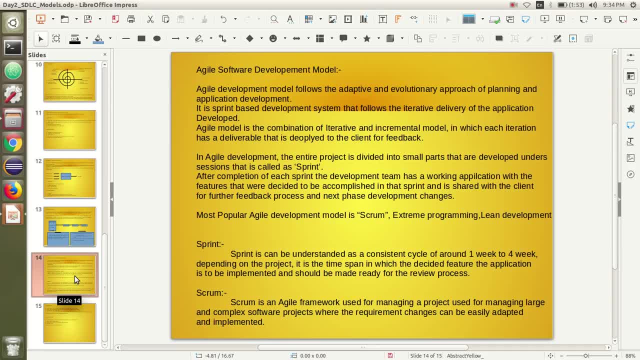 application development. it is a sprint based development system that follows the iterative delivery of the application developed. agile model is the combination of iterative and incremental model, in which each iteration has a deliverable that is deployed to the client for feedback and the development team is the one that is going to focus on the development of the project. 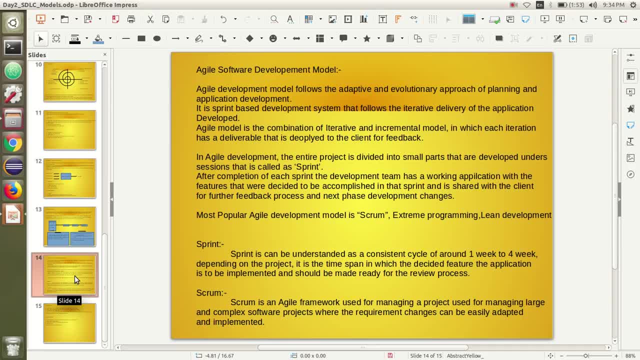 in agile development the entire project is divided into small parts that are developed under sessions. that is called sprint. so after completion of each sprint the development team has a working application with the features that were decided to be accomplished in that screen and is shared with the client for further feedback process and next phase development changes. 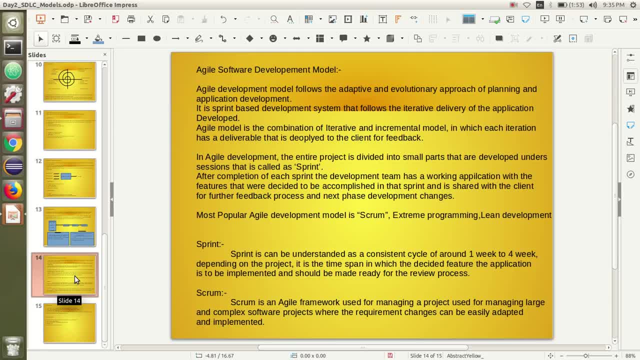 clear with the agile development model. like we have a particular time sprint in which we have, we have some predefined set of requirements that has to be implemented in within that sprint and the testing of that implementation should also be done within that sprint, and then that working model is deployed to the client for his review and feedback. 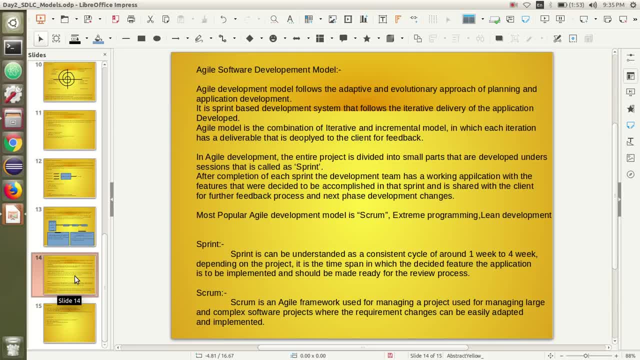 So mainly, Most popular agile development models are Scrum, Extreme programming, Lean development, etc. So let's understand some agile terminologies like sprint. So, guys, sprint can be understnded as a consistant cycle of around one week to 4 week, depending on a project. 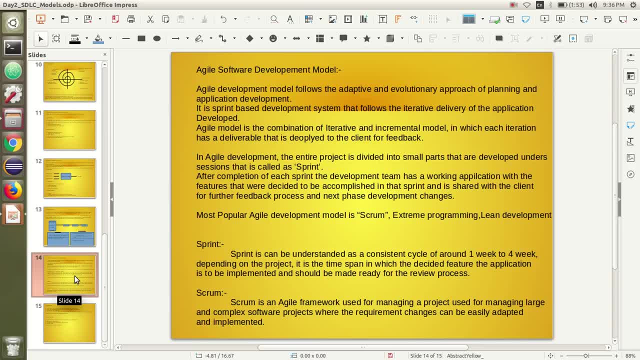 It is a time span in which the decided features, that that the decided features should be implemented in the application and should be made ready for the review process. so we can say that it is a time span of a week or or a month or of 15 days, it depends on the scrum. 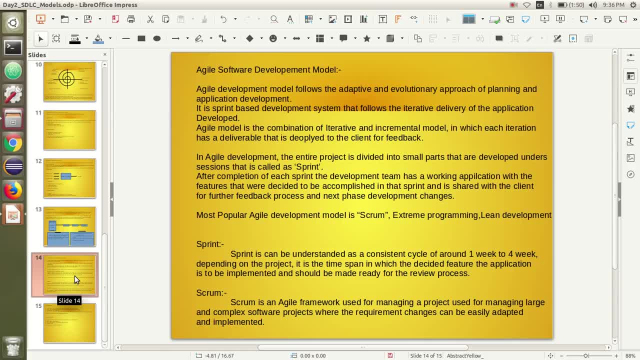 master or depends on the project, that on what kind of project you are working. so we have that particular time span in which we have to develop and implement the features that are discussed during the scrum meeting and that has to be implemented, implemented in the application, and that is to be. that has. 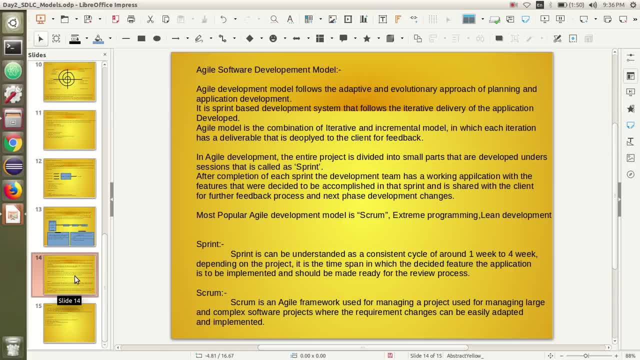 to be tested within that. that is print also, and after the completion of that screen, the application developed is deployed to the client for his review and feedback process. okay, so what is this scrum? scrum is an agile framework used for managing a project, used for managing large and complex software projects where the requirement changes can be easily. 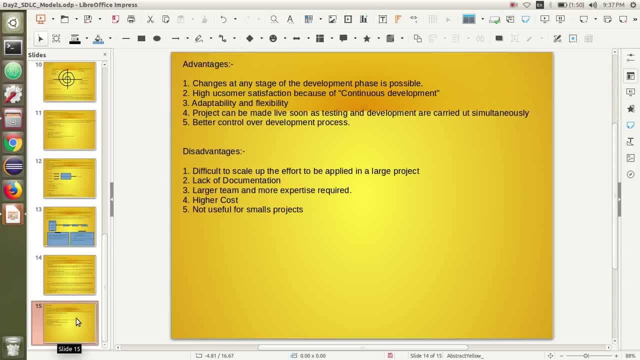 adapted and implemented. okay, so let's understand what are the advantages and disadvantages of using agile method for software software development. so advantages include changes in the configuration, quantity of software, the maximization of the Industries across the spectrum of Nebra or Alt5, and ones recommended implementation. can lead to a voting process. 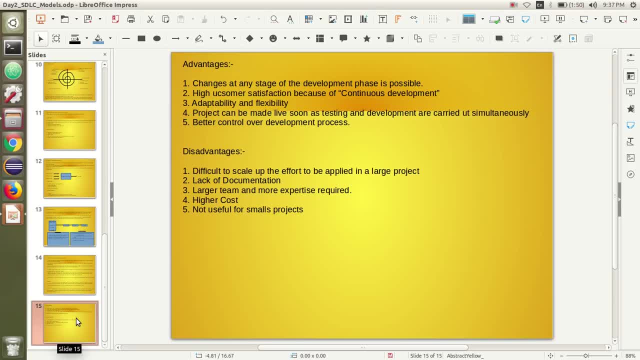 in the wal raj to your development level and bottom. quero se is very useful for our jakby find a solution really for this site. this is a very good use case so to fuel that. I am also very thankful to Prof X for giving us such a great opportunity with your help.